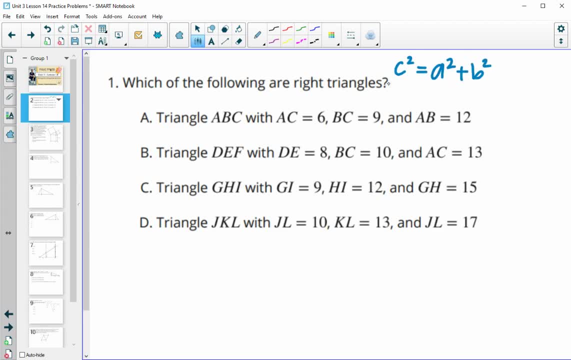 we plug them into Pythagorean theorem: see if both sides equal. So C squared needs to equal A squared and B squared added together, C is always the longer of the three lengths or the longest of the three lengths. So we see these three lengths, So we'll square them all. So 6 squared is 36,. 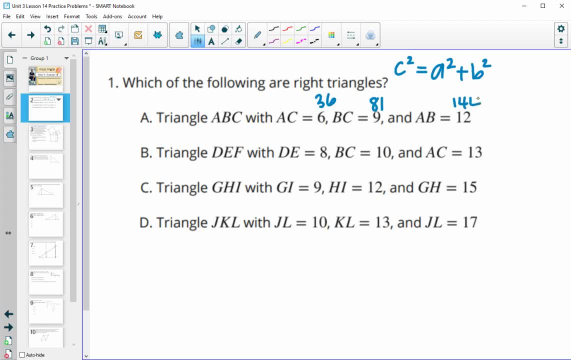 9 squared is 81, and 12 squared is 144.. And when we do 36 plus 81, that does not equal 144.. So this is not a right triangle. In part B, 8 squared is 64,, 10 squared is 100, 13 squared is 169.. So 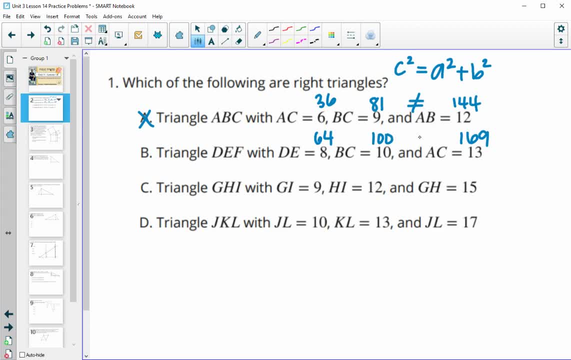 that's our C value squared, And 64 plus 100 does not equal 169.. So this is not a right triangle. In part C, 9 squared is 81,, 12 squared is 144, and 15 squared is 225.. 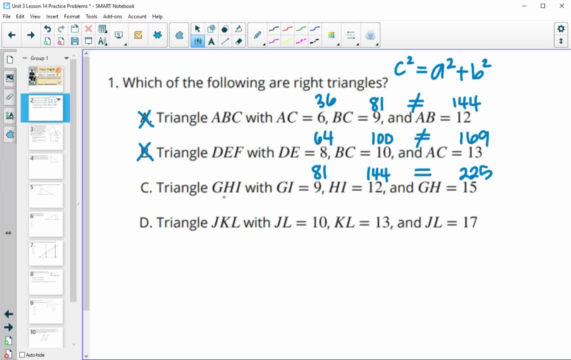 81 squared is 169.. So this is not a right triangle. 81 plus 144 is 225.. So these are equal to each other. So this one is a right triangle In part. D, 10 squared is 100, 13 squared is 169, and 17 squared is 289.. 100 plus 169. 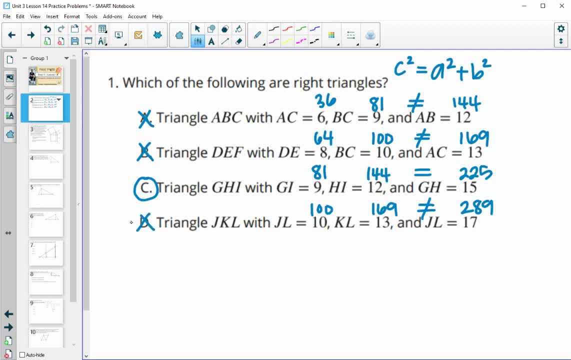 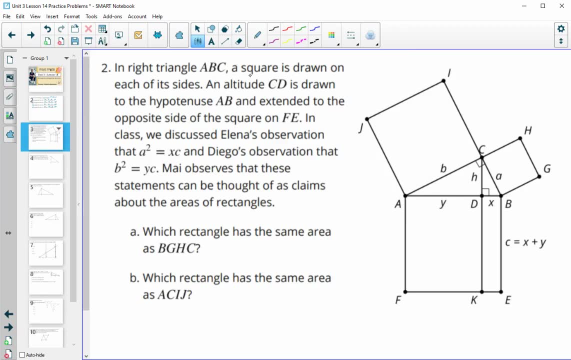 is not equal to 289.. So this is not a right triangle. Number two, in right triangle ABC, a square is drawn on each of its sides and altitude CD is drawn to the hypotenuse of AB from this right triangle and extended to the opposite side of the square, So the altitude is completely. 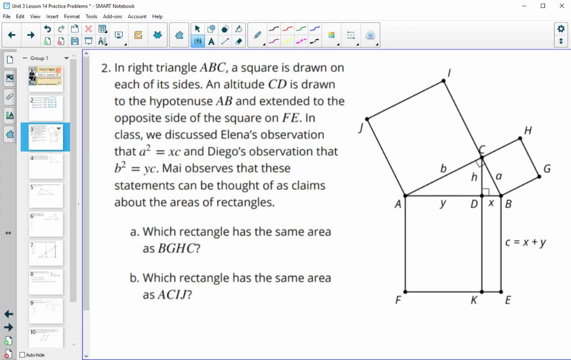 extended. here In class we discussed Elena's observation that A squared equals X times C And then Diego's observation that B squared equals Y times C. My observes that these statements can be thought of as claims about the area of the rectangles. So which rectangle has the same area as BCHG? So if we're saying this little triangle here, 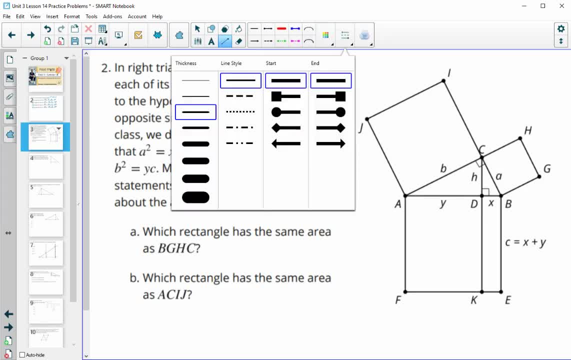 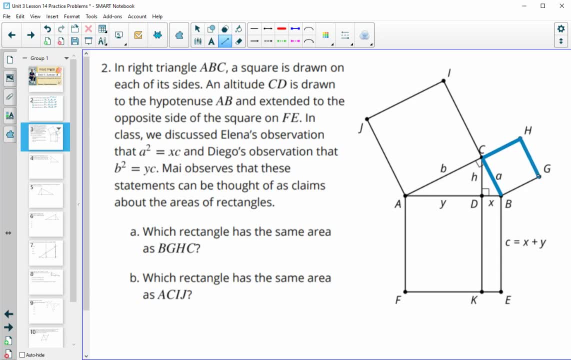 let me get some color here to help us look at it. So this is side length is A. So then this square here has side lengths of A, So all the side lengths are A. So then this area would be A squared, A times A. And then we see that Elena said that A squared is equal to X times C. 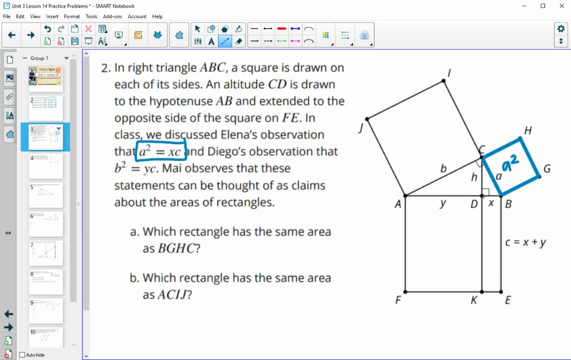 So which rectangle is that? And so we see here's an X and then here's side, length C. So this rectangle's area would be XC. So the area of this would be X times C, which is what Elena is saying- is equal to A squared. 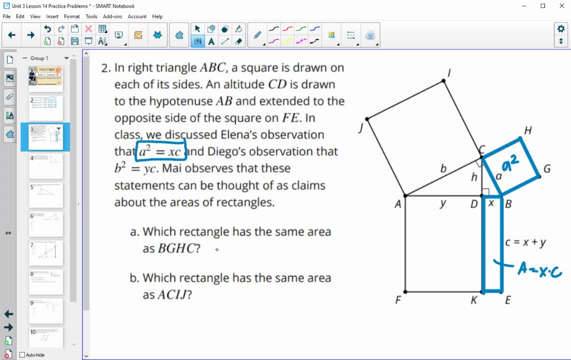 So these two blue rectangles would have the same area, So B, E, K, D for this one. And then what about the other rectangle? So what about equal to the rectangle A, C, I, J? So this orange triangle, or this orange rectangle, is this one. 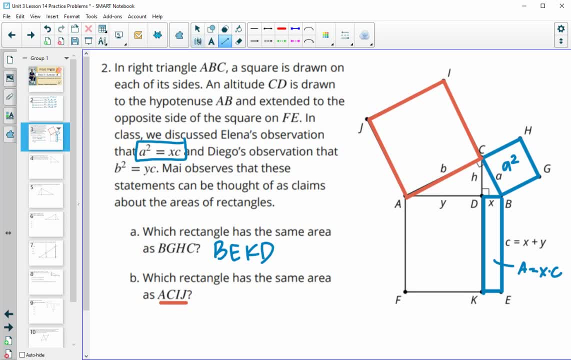 So which of the other rectangles has the same area as that one? And so the area of this one. each of these sides are B's, So the area of this is going to be B squared. And then we remember that Diego said that B squared equals Y times C, And so Y times C, here's Y. And then remember that this length 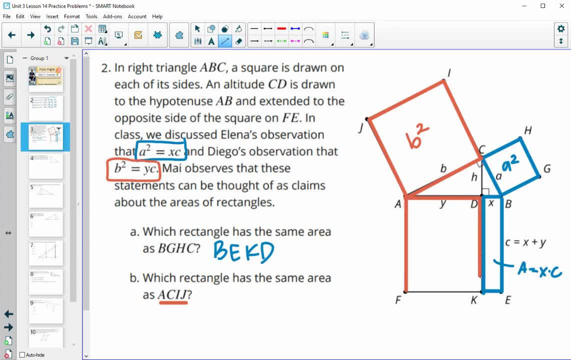 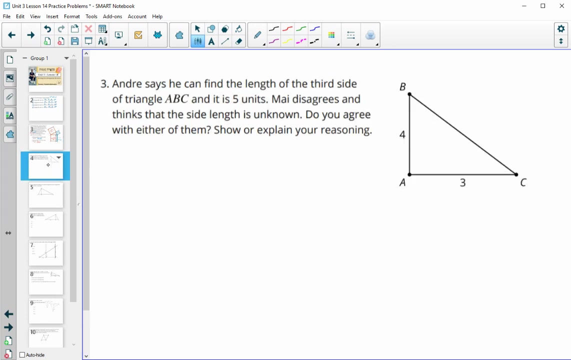 is C. We see it right here. So this rectangle here is equal to the area, is equal to Y times C. So then we're saying that B squared is equal to Y times C. So these two rectangles would have the same area. So ADKF Number three: Andre says that he can find the length of the third. 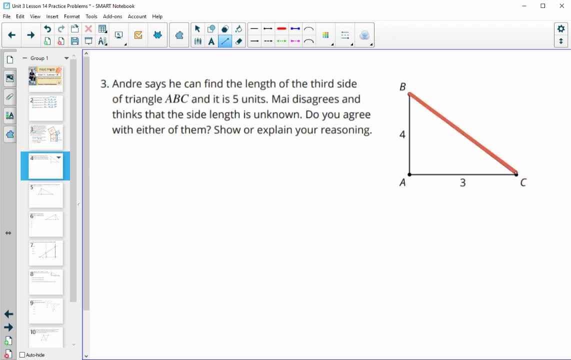 side in triangle ABC And he says that it is five units. So he's saying he can figure this out as five units. Mai disagrees And she thinks that the length of the segment is unknown. So do you agree with either of them and explain your reasoning? All right, So it would be five units if we knew that. 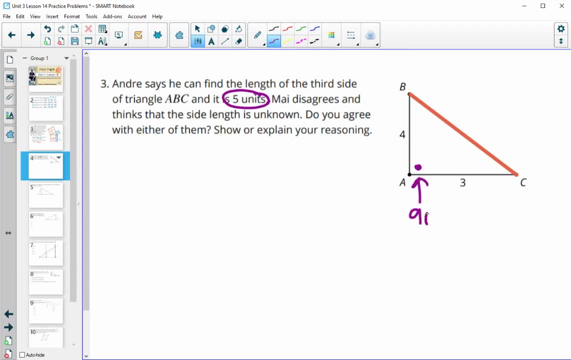 this was a right angle. Okay, We need to know that this is a 90 degree angle, And without that, then this is an unknown segment. So when we don't know that it's 90 degrees, then we can't do anything else. If this were a 90 degree, 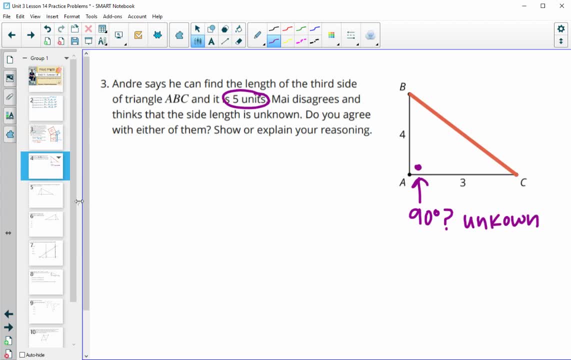 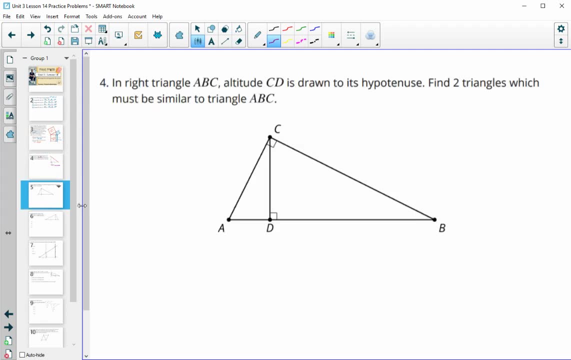 angle, then we would be able to do Pythagorean theorem. Without the 90 degree angle we can't do anything. So agree with Mai. Number four: in a right triangle ABC, the altitude CD is drawn to the hypotenuse. Find two triangles that must be similar to triangle ABC. 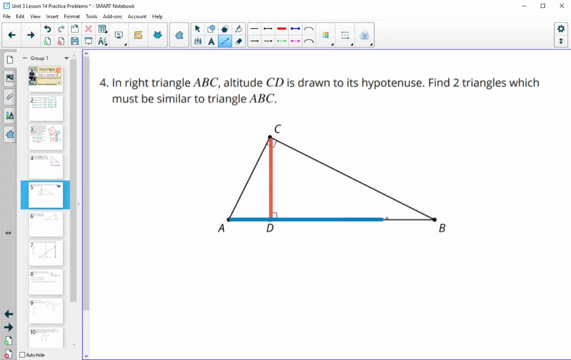 So here's triangle ABC. So A to B to C, And remember that that order matters. So when we did this triangle here, okay, we went from A to B, which is the hypotenuse, and then B to C, which is the long leg, And then we went to the short leg. So I'm just going to leave it like this. 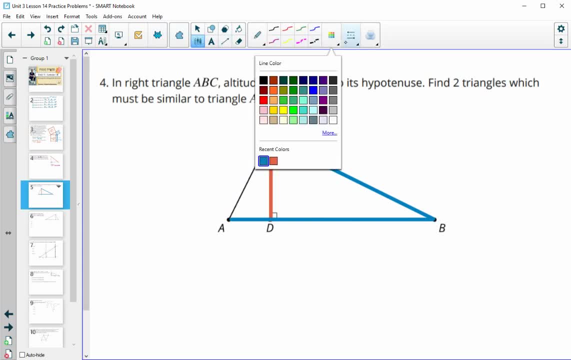 so we remember the order that we're going in. So A to B to C. So we need to follow the hypotenuse To the long leg in our letter orders. So we want to come up with two triangles that are similar to ABC. I'm actually going to delete this hypotenuse out of here, All right. so these two little 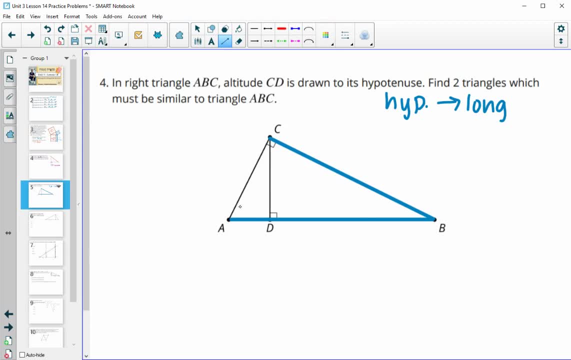 triangles are going to be similar to the larger one And again we just have to follow hypotenuse to long leg. So in this little triangle over here, if I go hypotenuse to long leg, the order of those letters is A to B to C. So we're going to have to follow hypotenuse to long leg. So in this little 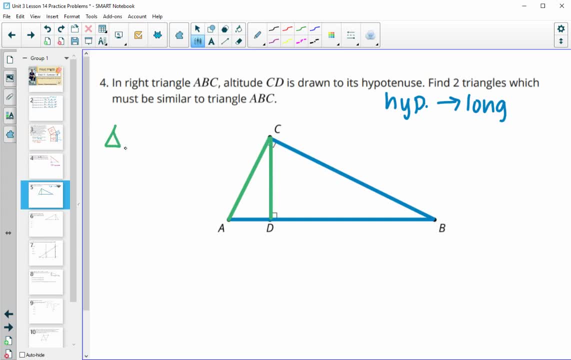 triangle over here. if I go hypotenuse to long leg, the order of those letters is A, C, D. So triangle A, C, D is similar to ABC. And then if we do it again in this kind of medium-sized triangle, 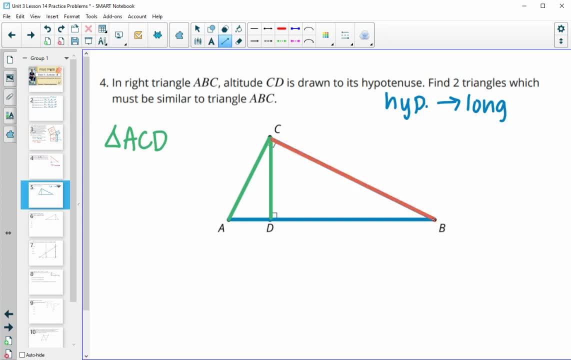 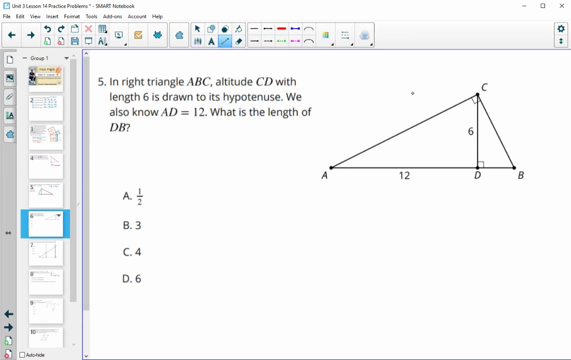 over. here we need the hypotenuse to the long leg. So the letter of those orders are C, B, D. So then triangle C, B, D is also similar to triangle ABC Number five in right triangle ABC, the altitude C D is the altitude and it has a length of six. 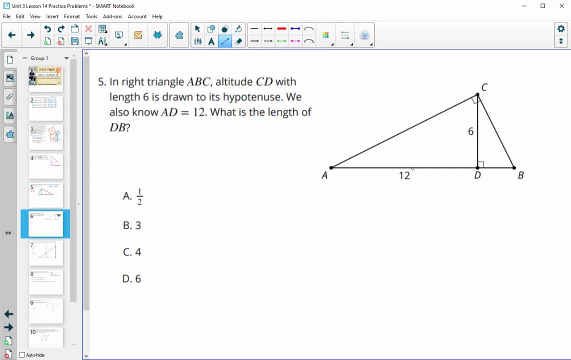 so we can see that. And then we also know that A, D is 12. What is the length of B D? So we want to find this segment here, So we know that the hypotenuse kind of pieces here split up. 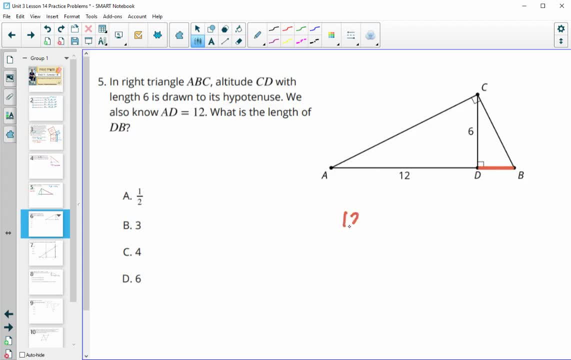 are proportional with the altitude, So we can take 12, over 6.. So 12 over 6 is going to be equal to 6 over this missing piece here of BD, and then we'll be able to cross multiply. So if we multiply BD up, we get 12 times BD, equals 6 times 6, which is 36. 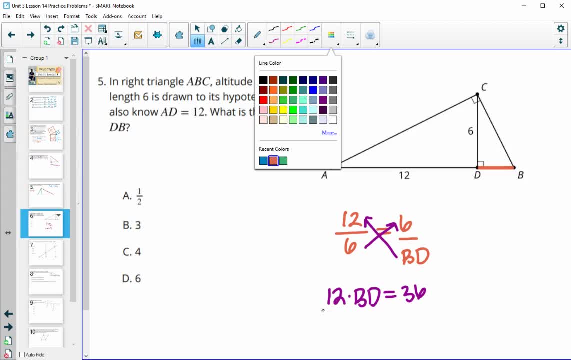 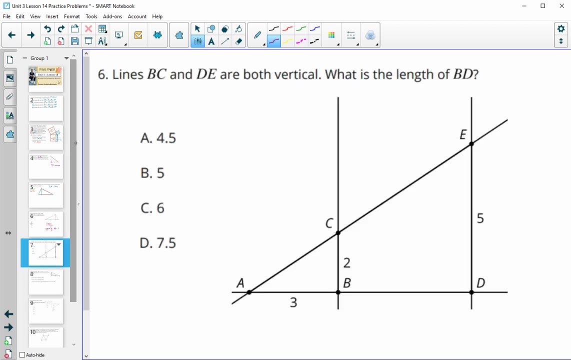 and then we will divide both sides by 12 and we end up with: BD is equal to 3.. Number six, BC and DE are both vertical, so when we have two vertical lines, we know that that means that they're parallel, which also splits these sides up proportionally and gives us 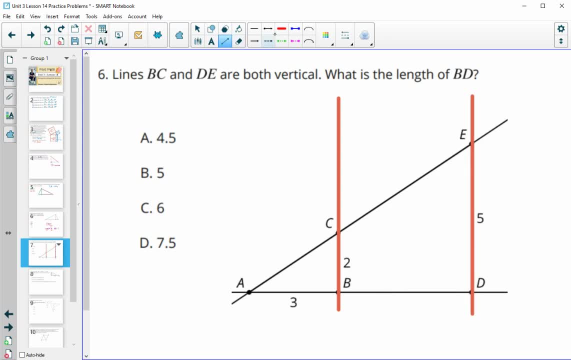 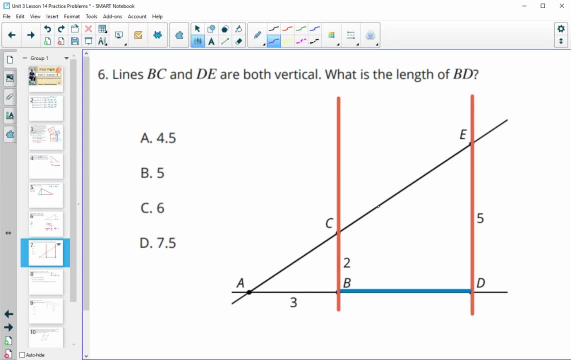 and we don't have these other side pieces over here, so we're going to have to use the similar triangles to figure this out. and so if we take a look at this little green triangle and then we compare that to this larger triangle here, so this one- 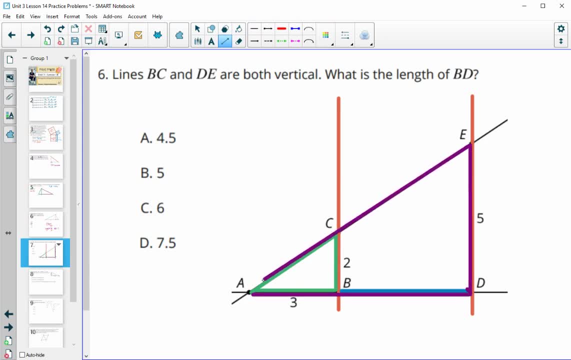 we'll be able to find the length of segment AD and then that will help us get to BC. So we've got this. two is this side and the five. so we'll compare those with scale factor. So the scale factor is five divided by two or 2.5. so we multiply by 2.5 to get to that larger side. So we'll do that with. 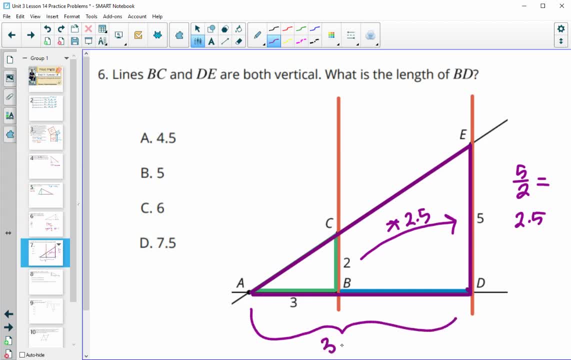 this one to get AD. So we'll take this one and we'll compare those with scale factor. So we'll take three times 2.5 and that's going to give us 7.5 for AD Then to get this little missing piece. 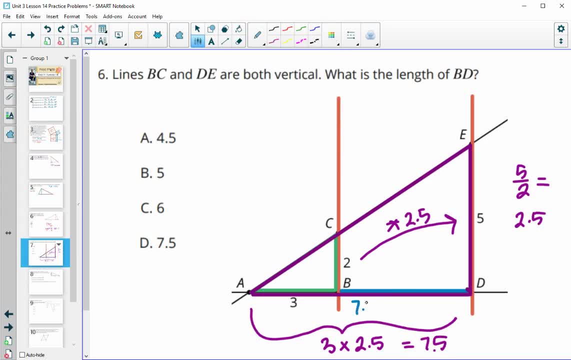 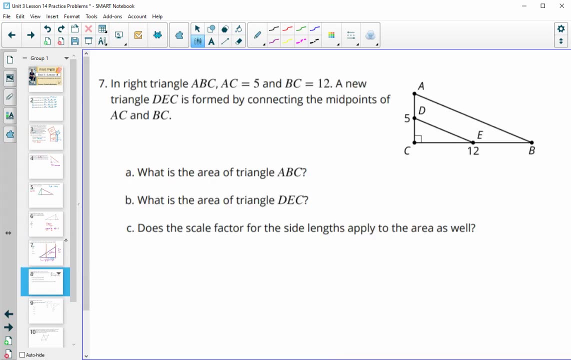 here. so all we want is from B to D. so we're going to take 7.5 minus the three that we've already used here, and we'll get 4.5 for segment BD, Number seven, BD. in this right triangle we see that AC is 5 and BC is 12, and then a new triangle is formed by 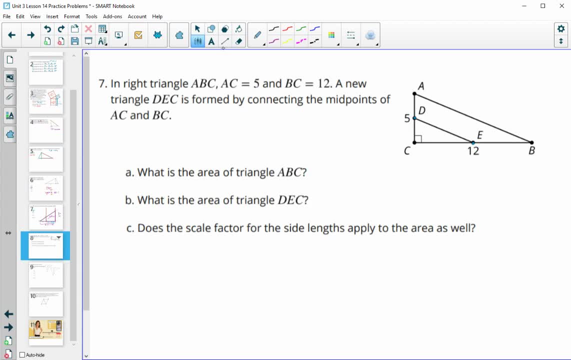 connecting the midpoints. so these are the midpoints. let's figure out the area of triangle ABC. so ABC is this larger triangle. and remember to figure out the area, we do base times height divided by 2. so we'll do 5 times 12 divided by 2, and 5 times 12 is 60, divided by 2 is 30 units. 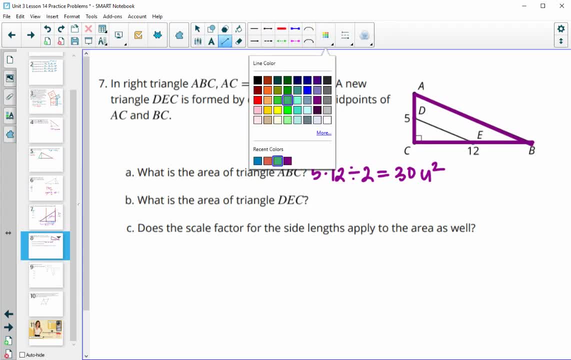 squared, then we'll figure out the area of triangle DEC. so DEC is this little triangle here formed by the midpoints. so we know with this one that this side is half of AC, so this is 2.5 and this one is half of 12. So this one is 6.. So we will do 2.5 times 6 divided by 2, and we get 7.5 units squared. 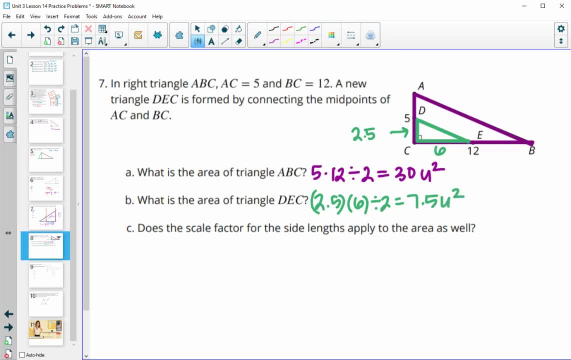 for that triangle. Now this last question says: does the scale factor for the side lengths apply to the area as well? So let's look at the side length factor. Okay, so the side factor is comparing a new length. So let's compare 2.5 to the original length of 5. And so we know that that equals down. 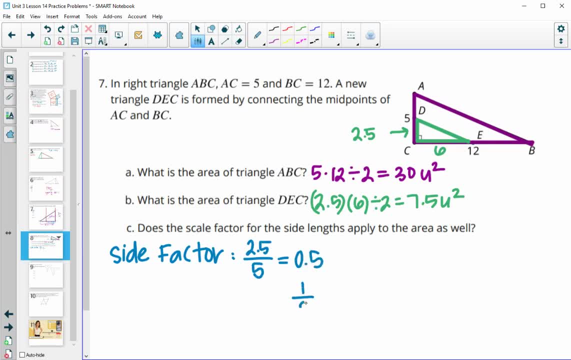 to a decimal of 0.5 or a fraction of one half. So there's our side scale factor. Then let's look at our area factor and see if it's the same. So our area will again take the new area of 7.5 and compare that to the original area of 30.. 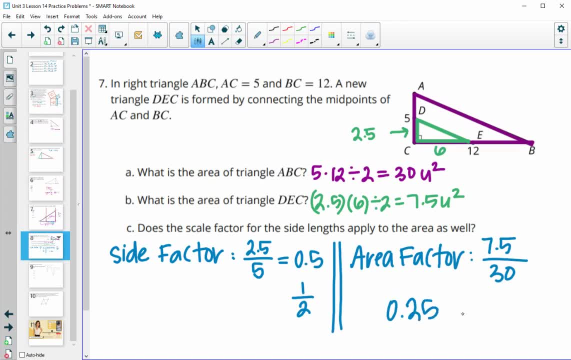 And we see that this divides down to a decimal of 0.25, or a fraction of one fourth, And we see that those are not equal. So one half does not equal one fourth. So the side and area factors are not equal or they do not apply. 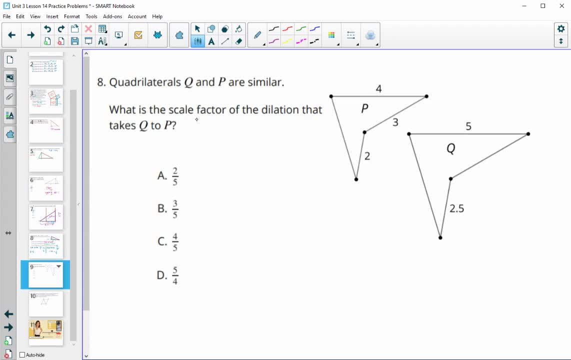 Number eight quadrilaterals. P and Q are similar. What is the scale factor that takes Q to P? Okay, so our new shape is P. So we'll take a measurement in P divided by the original in Q and we get a scale factor of four fifths. Let's say you had compared these ones because 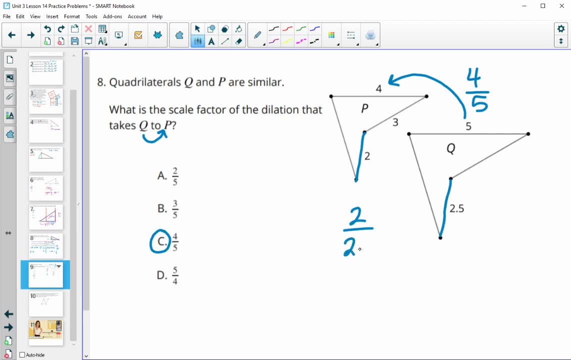 you can do that as well, And then you would have just gotten 2 divided by 2.5.. You wouldn't see that here, You wouldn't see that exact fraction, So you could just try again with a different set. or you could just try again with a different set. So you could just try again with a different set. 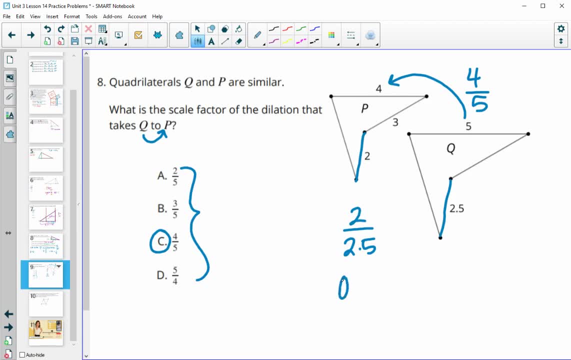 You could divide this down and do 2 divided by 2.5 and get 0.08, and then divide all of these And for this one you'd have gotten 0.04 or 0.6, and then you would have gotten to 0.8 here. 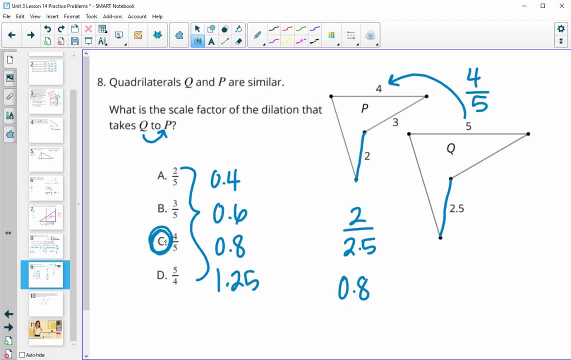 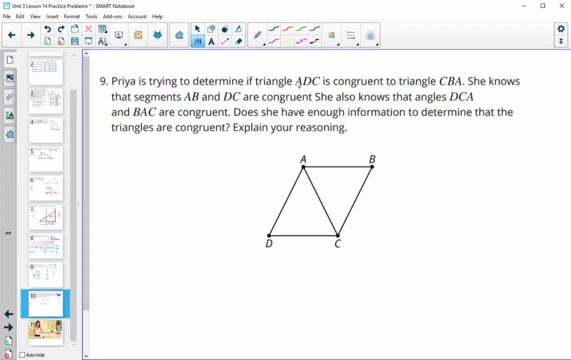 and 1.25 here and that would have helped you to have seen C as well. Number nine, PREA, is trying to determine if triangle ADC- okay, so this one down here- congruent to CBA, so this one up here. She knows that segments AB and DC are congruent, So AB is. 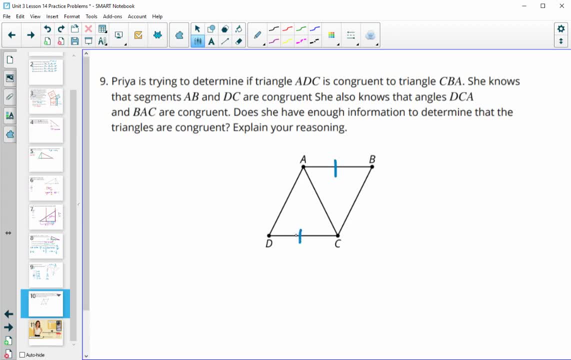 congruent to DC. She also knows that angle DCA. so this angle here is congruent to angle BAC, this angle here. Does she have enough information to determine that the triangles are congruent? Explain your reasoning. So that's the stuff that she was given, PREA also. 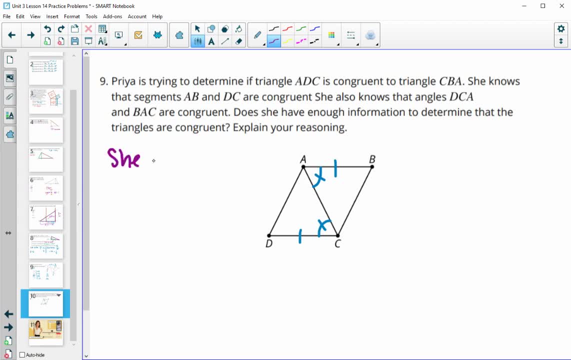 knows that, so she also knows that AC is congruent to CA. So AC kind of in this bottom triangle and CA in this top triangle are congruent because they are the same segment, which is the reflexive property, And then this gives her enough information. Okay, so then she knows the triangles are.